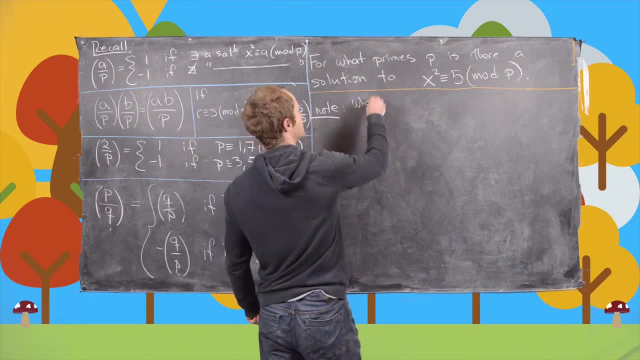 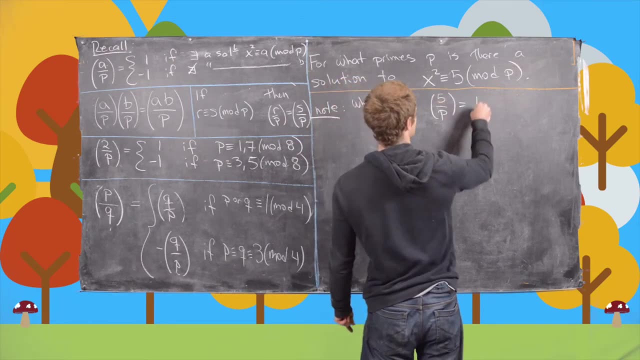 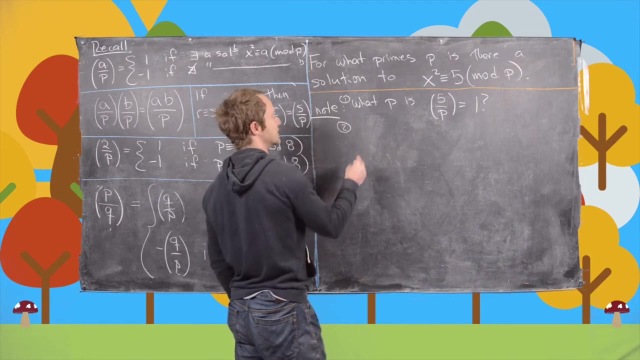 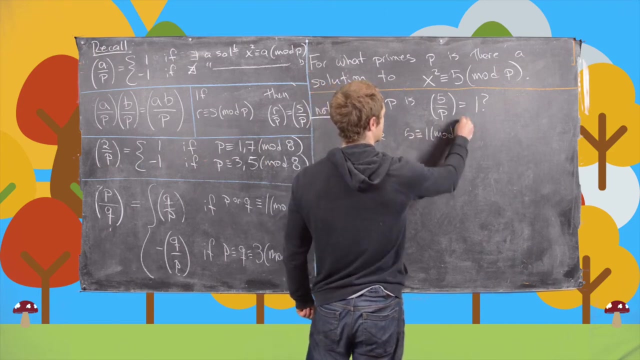 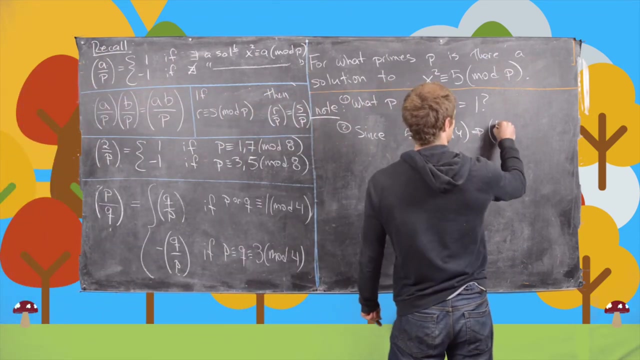 question for what p is? 5 by p, this Legendre symbol equal to plus 1.. Okay, good, maybe that's the first thing to notice. And then the second thing to notice is, since 5 is congruent to 1 mod 4, we can apply this property of quadratic reciprocity to tell us that 5 by p is the same. 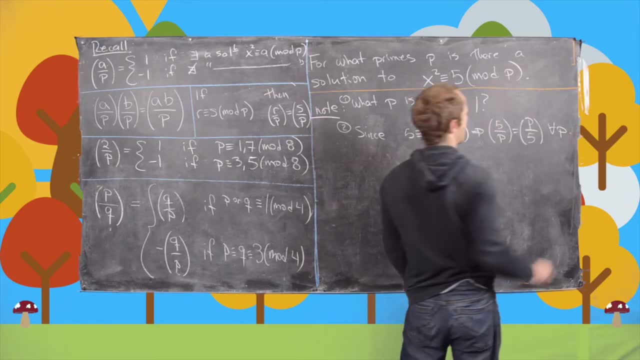 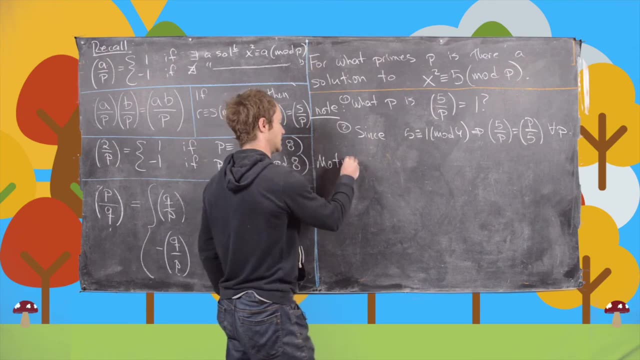 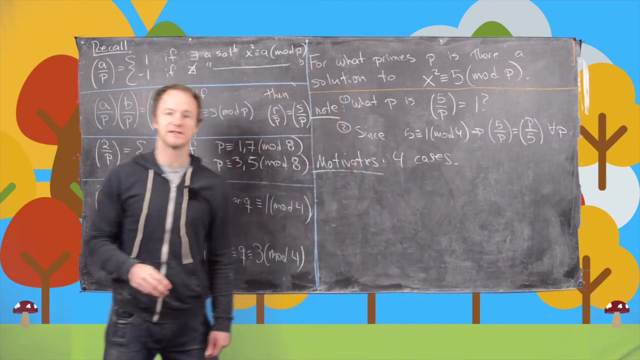 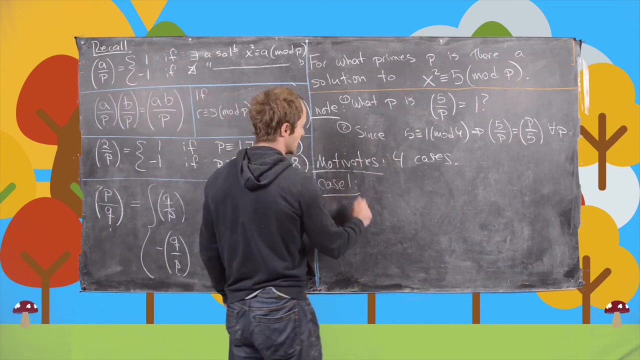 thing as p by 5 for all primes p. Okay, good, and now that motivates everyquisite problem here. So let me go back and see what I have on here and let's go ahead and look at case 2. Canyon law 😅. So for case 2 we have four cases and those cases are all of the 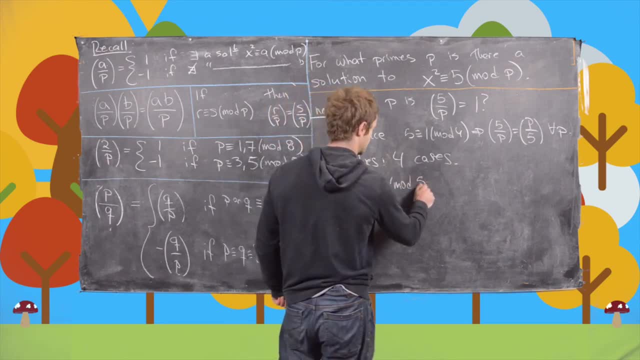 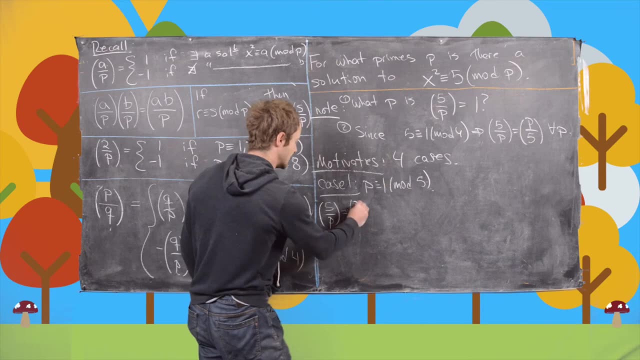 residues modulo 5.. And so we'll do these one case at a time. So case number one: we'll look at if p is congruent to 1 mod 5.. Good, So, if p is congruent to 1 mod 5, we have 5 by p, is p by 5.. But now, since p is ninetstrual, 5. We've got 2 times Everyquisite problems. Also, right now, shape the problem if 3.. neighbors лемinism, there is nocas CR G Matter right now. otherwise 2, yeah, very specific, because bathroomери can't get along here. when we have division, we can't see each one three. 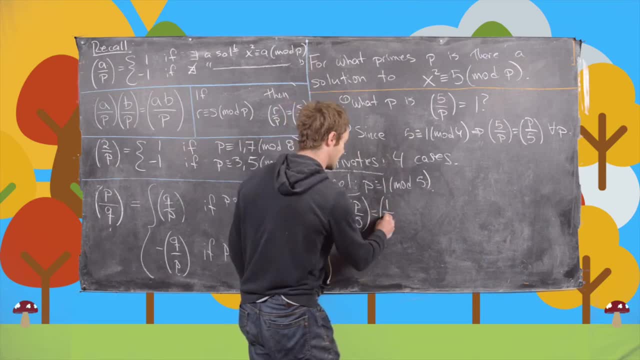 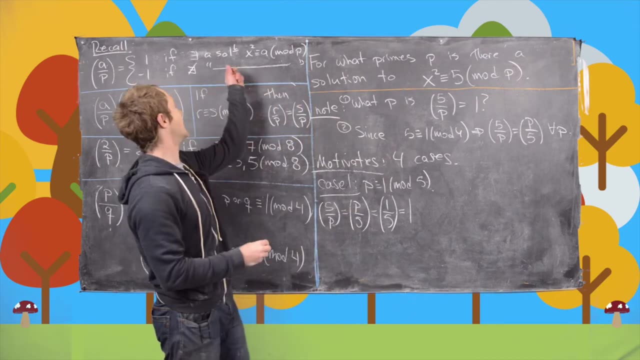 because here case number 1 can't get along with it. One can't get along with each. p is congruent to 1 mod 5, we get 1 by 5, but then that's obviously equal to 1, and that's because 1 squared is equal to 1.. There's obviously a solution to this equation, Okay. 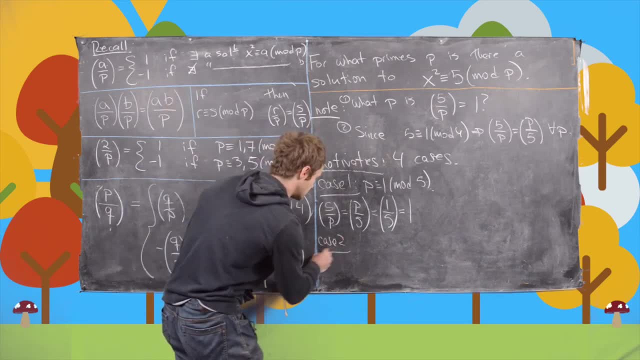 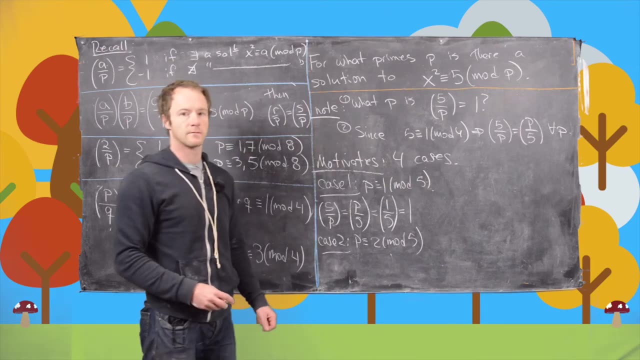 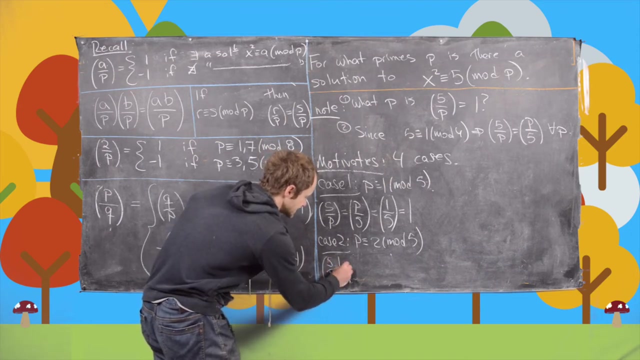 good, So now let's look at case 2.. So we have: p is congruent to 2 mod 5.. Okay, so now for the second case. we have: 5 by p is the same thing as p by 5, and then by this equivalence. 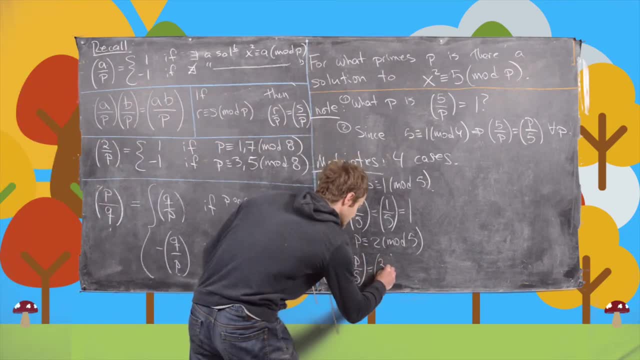 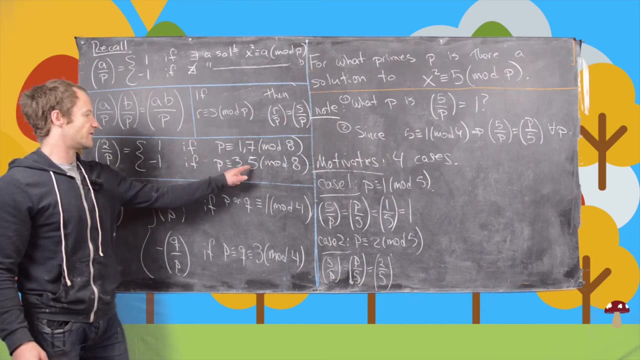 and this property right here we have. that's the same thing as 2 by 5, but now 5 is a prime of the form 5 mod 8. In fact it's 8 times 0 plus 5, so that tells us that this is negative.